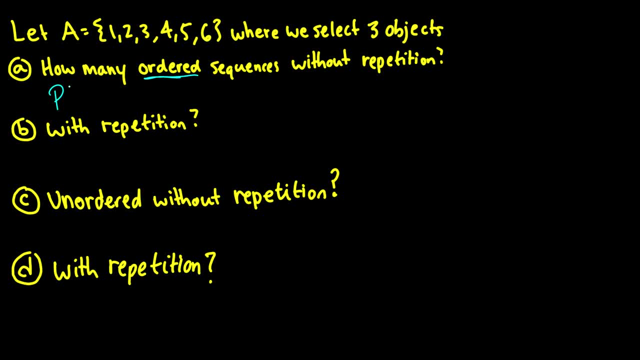 so we have P, there are six total objects, and we have to choose three. Now, if this isn't satisfying for you, well, the first object can be picked six ways, the second object can be picked five ways and the third object can be picked four ways. So that is a way of looking at it. What about with repetition? Well, that just means that for each object we pick, we have six of. 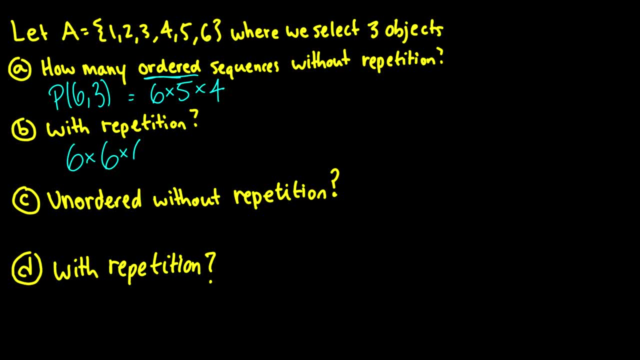 available choices. So this is going to be six times six times six, which is equal to six cubed. Okay, now let's go to the unordered section. So these are combinations and without repetition. Well, we know that this is just six choose three, a very simple operator, And this is actually a completely sufficient answer. Now we're going to. 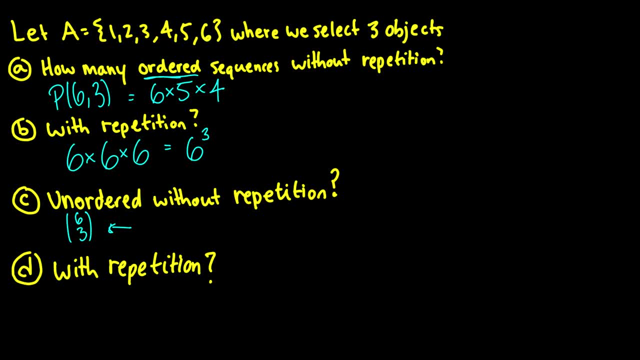 with repetition. if you don't remember, the formula might be a little bit trickier, But if you do remember it is n plus r, minus one. choose r, where n is the total number of objects you have available, which is six, and r are the amount of objects you're selecting, which would be three. So if you pick it with repetition, unordered, you are going to have eight. choose three. 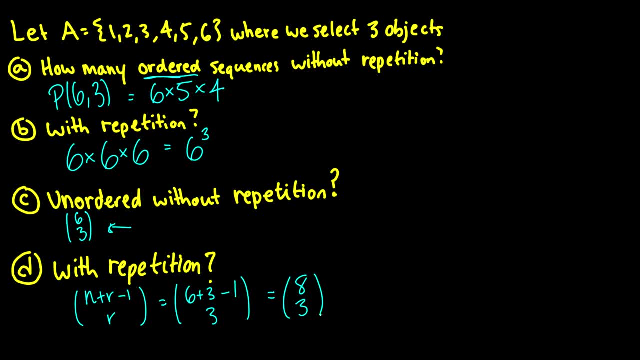 So these first four questions are really just: did you remember the formula? Because they're pretty basic, the numbers are very easy to work with And you can probably. if you honestly didn't know how to do this, you could probably list all the different possibilities in 10 minutes for all of these, So it's really not that bad. 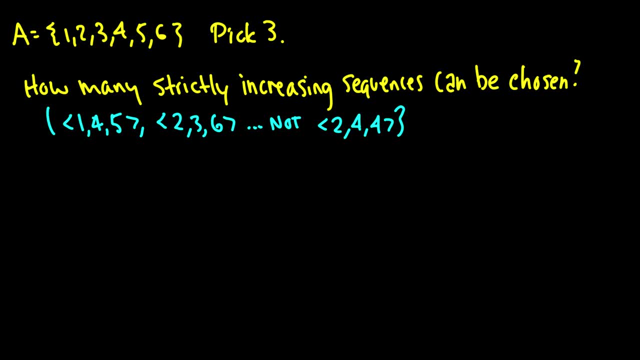 So we have the same problem as the first question, But now we're going to make it a little bit more challenging by saying how many strictly increasing sequences can be chosen. And this is where the second number is always greater than the first and the third number is always greater than the second. So two, four, four is not acceptable because this last four is not strictly greater than the previous number. 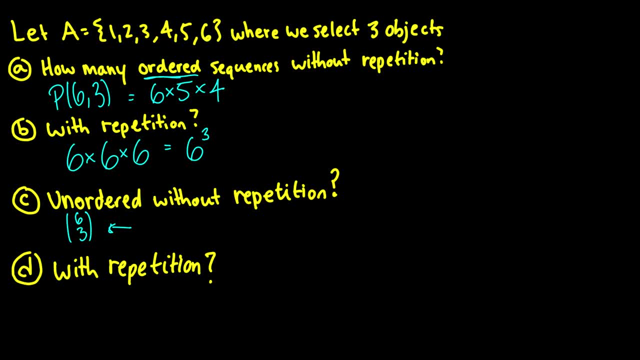 with repetition. if you don't remember, the formula might be a little bit trickier, But if you do remember it is n plus r, minus one. choose r, where n is the total number of objects you have available, which is six, and r are the amount of objects you're selecting, which would be three. So if you pick it with repetition, unordered, you are going to have eight. choose three. 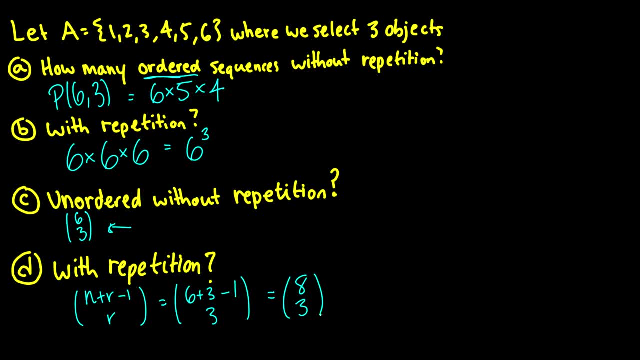 So these first four questions are really just: did you remember the formula? Because they're pretty basic, the numbers are very easy to work with And you can probably. if you honestly didn't know how to do this, you could probably list all the different possibilities in 10 minutes for all of these, So it's really not that bad. 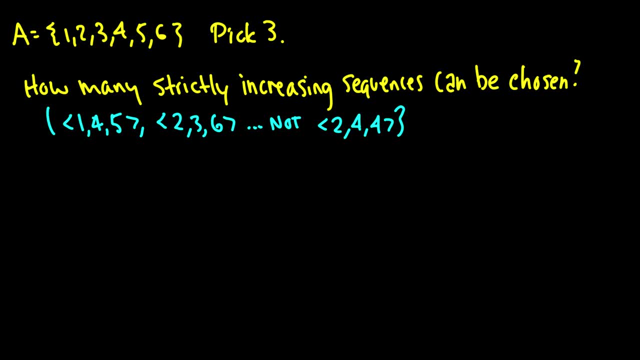 So we have the same problem as the first question, But now we're going to make it a little bit more challenging by saying how many strictly increasing sequences can be chosen. And this is where the second number is always greater than the first and the third number is always greater than the second. So two, four, four is not acceptable because this last four is not strictly greater than the previous number. 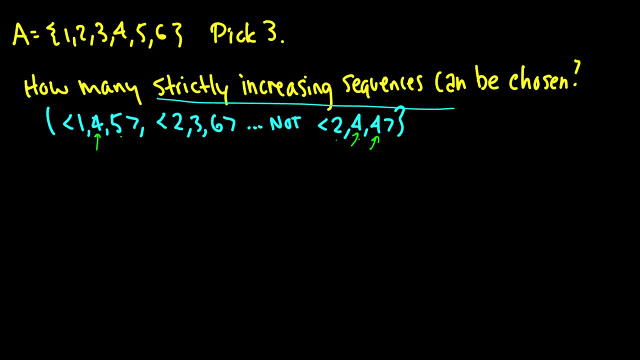 I want you to answer this on your own right now, because I will give you the answer and then explain how to do this. Okay, so hopefully you took some time to figure it out. The correct answer is just six, choose three. Now this may seem unintuitive, but it's pretty obvious, and I'm going to show you why. 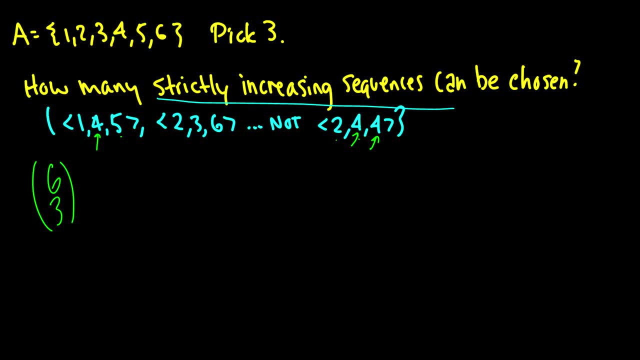 So say, we have the numbers four, One and two. Well, we know this is the same thing as one, two, four, which is strictly increasing. So what we do is we say, okay, let's do six, choose three and then order them. 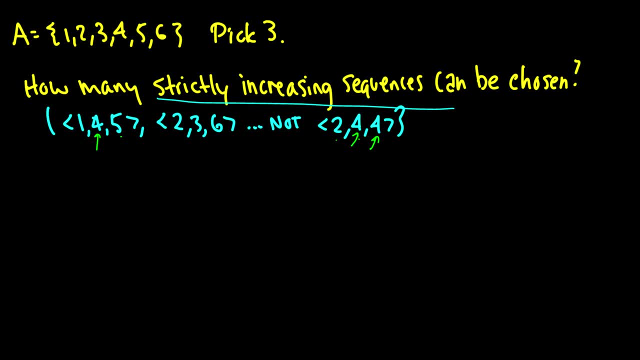 I want you to answer this on your own right now, because I will give you the answer and then explain how to do this. Okay, so hopefully you took some time to figure it out. The correct answer is just six, choose three. Now this may seem unintuitive, but it's pretty obvious, and I'm going to show you why. 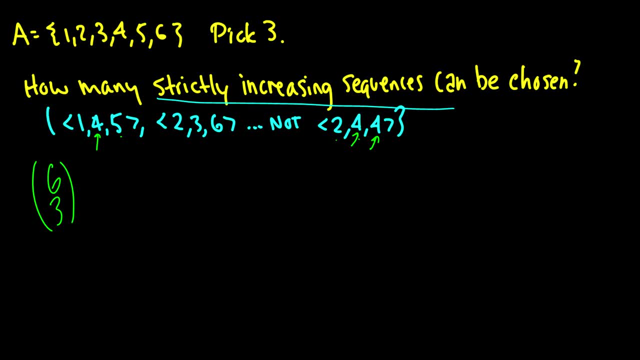 So say, we have the numbers four, One and two. Well, we know this is the same thing as one, two, four, which is strictly increasing. So what we do is we say, okay, let's do six, choose three and then order them. 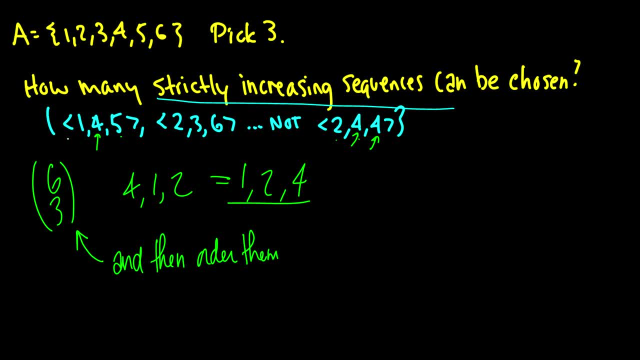 So I know these are ordered pairs here- one, four and five- but it never says we have to order them first and then pick them. Why don't we pick them and then order them? And we know that in six, choose three. there's not going to be any repetitions of numbers. 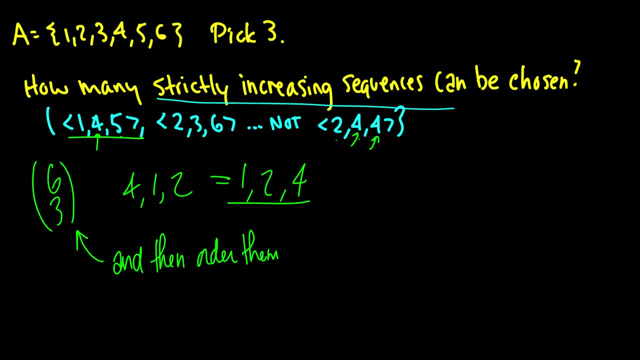 So once you order them, they are always going to be strictly increasing. Now, what if I said: how many strictly decreasing sequences are there? So let's change increasing to decreasing. Now what happens? What is the new answer? Well, the new answer again is just six. choose three. 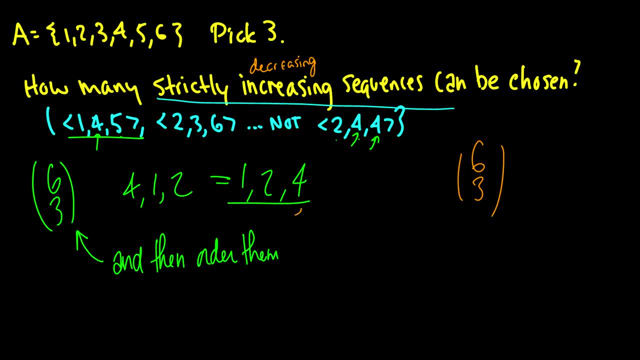 Okay, We just reverse the order and it's exactly the same. If we were to say how many just, instead of strictly how many increasing sequences there were. so one, two, four, four would be acceptable. then it would be eight. choose three, because 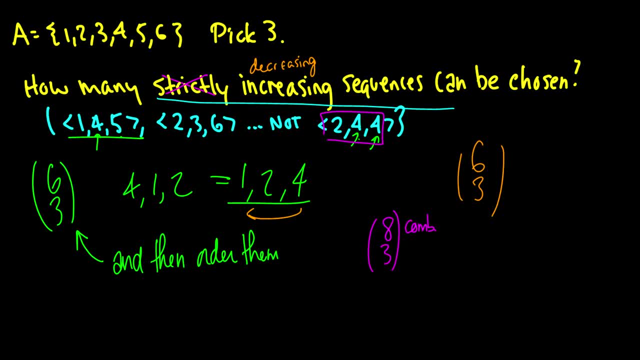 all this is is combinations with repetition. Okay, So this question is designed to fool you and make you think and to find an answer that is much more complicated than it necessarily has to be. Anyways, we've got one more question here. 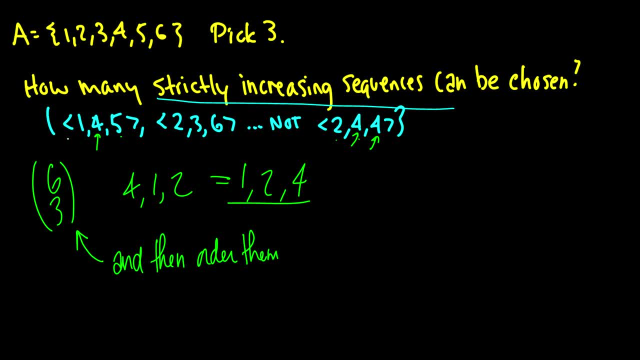 So I know these are ordered pairs here- one, four and five- but it never says we have to order them first and then pick them. Why don't we pick them and then order them? And we know that in six, choose three. there's not going to be any repetitions of numbers. 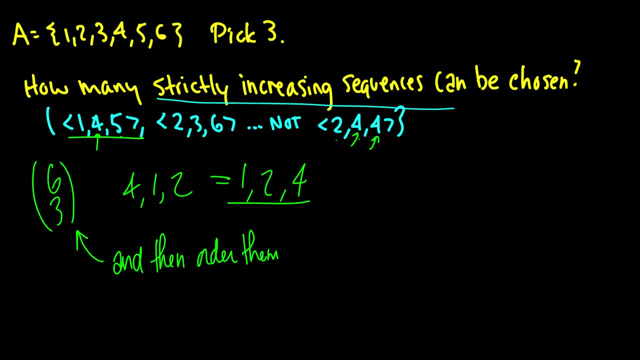 So once you order them, they are always going to be strictly increasing. Now, what if I said: how many strictly decreasing sequences are there? So let's change increasing to decreasing. Now what happens? What is the new answer? Well, the new answer again is just six. choose three. 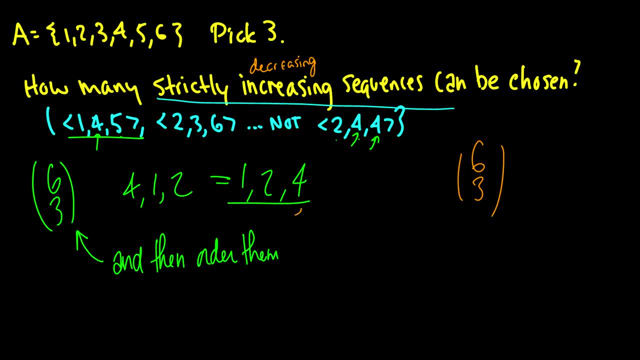 Okay, We just reverse the order and it's exactly the same. If we were to say how many just, instead of strictly how many increasing sequences there were. so one, two, four, four would be acceptable. then it would be eight. choose three, because 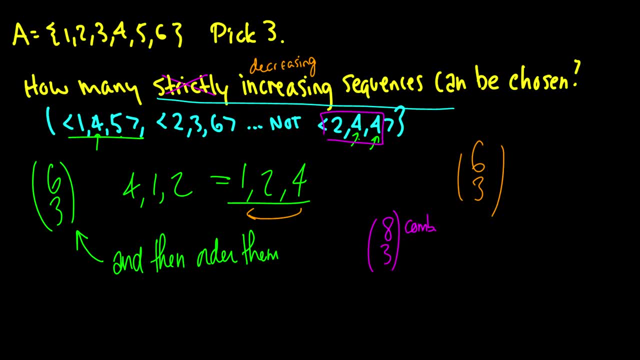 all this is is combinations with repetition. Okay, So this question is designed to fool you and make you think and to find an answer that is much more complicated than it necessarily has to be. Anyways, we've got one more question here. 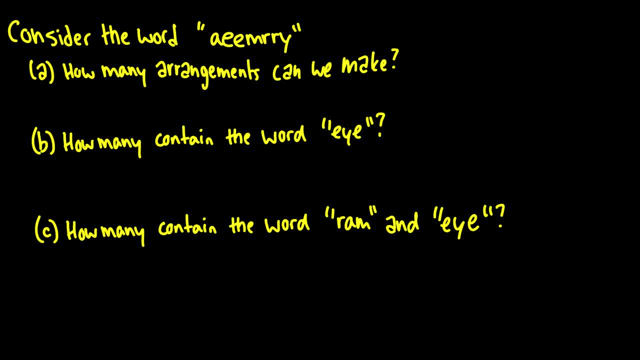 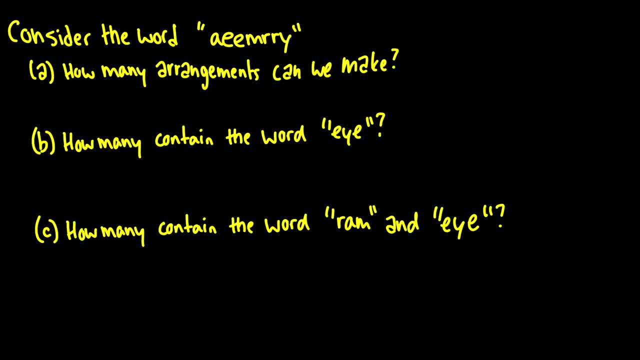 But here's the question: How many arrangements can we make? Well, if you remember before, first we have to take the amount of numbers or letters there are, which will be seven. So we take seven factorial and then we divide it by however many duplicates there are. 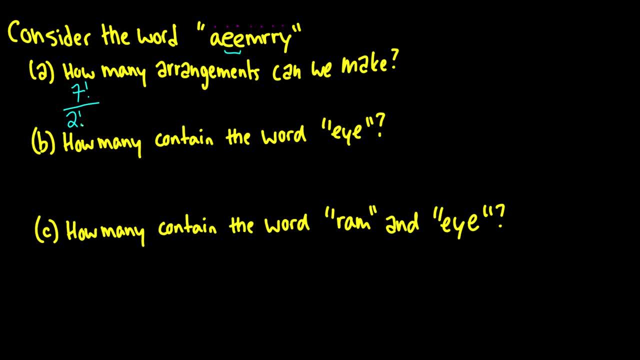 So there's two e's, so we divide by two factorial and there's two r's, so we also divide by two factorial, Two factorial, And this will be our answer. So that wasn't too bad. But here's a better question. 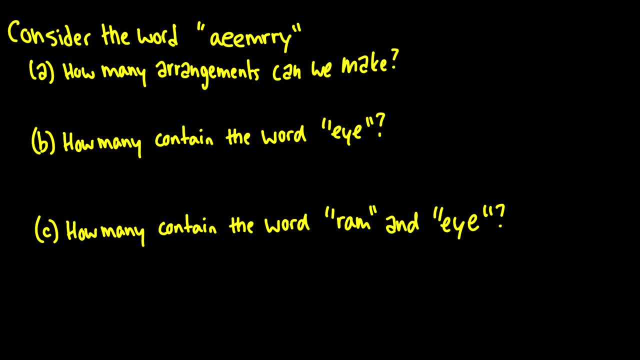 Consider the word a-ree. I am sure this could have been a fake word, like memery or something, But I guess the vowels and letters are separated for convenience. But here's the question: How many arrangements can we make? Well, if you remember before, first we have to take the amount of numbers or letters there. 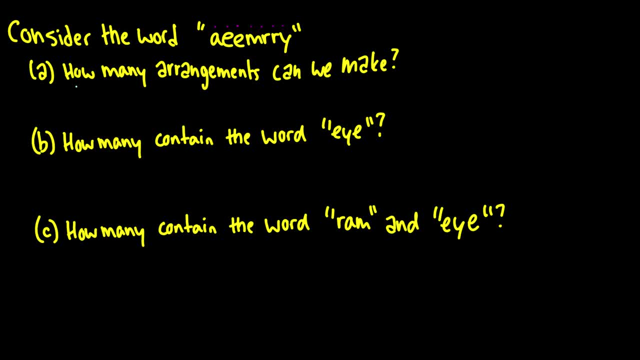 are, which will be seven. So we take seven factorial and then we divide it by however many duplicates there are. So there's two e's, so we divide by two factorial, and there's two r's, so we also divide by. 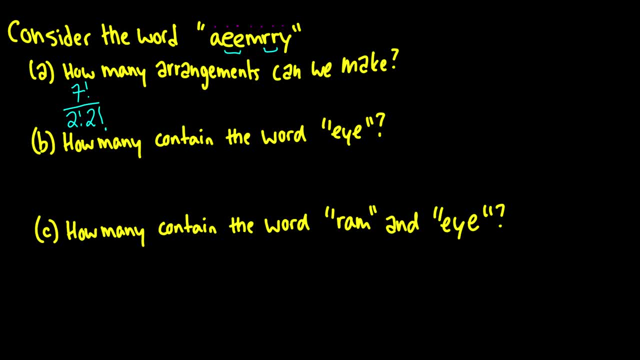 two factorial, And this will be our answer. So that wasn't too bad. But here's a better question: How many contain the word I? Well, now, what we do here is we take our word out. So let's take the word I out and then list the remaining letters here. 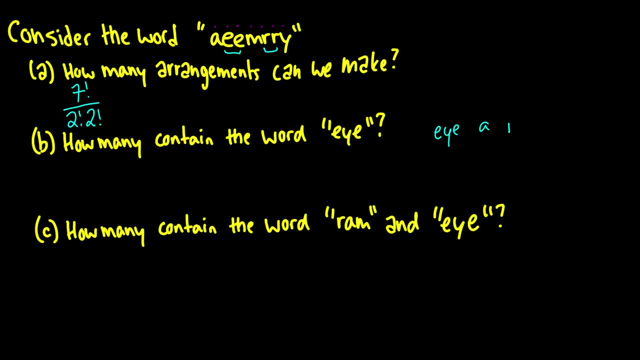 We have A, we have an M and we have two r's. So what we do is we treat the word I Okay, So we take the word I as a single element. So now we actually have one, two, three, four, five total elements here. 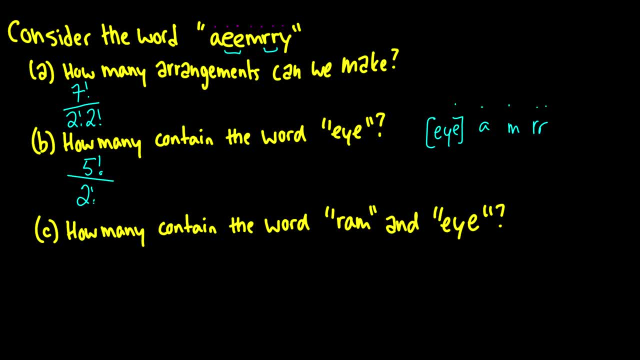 And how many repeats are there? Well, there are two r's, So this is five factorial over two factorial. So I know this might seem a little bit confusing, but essentially we just combine the letters EYE into one element and then do the rest as normal. 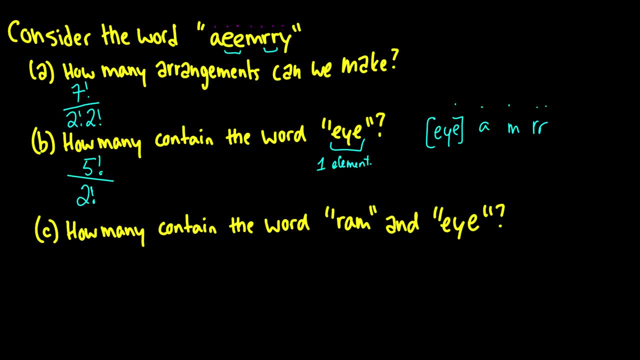 In fact, if you were to take the total arrangements and then subtract all the arrangements where EYE happened to be together with much more complicated mathematics, you would end up at this same result if you did it correctly. So here's a better question. 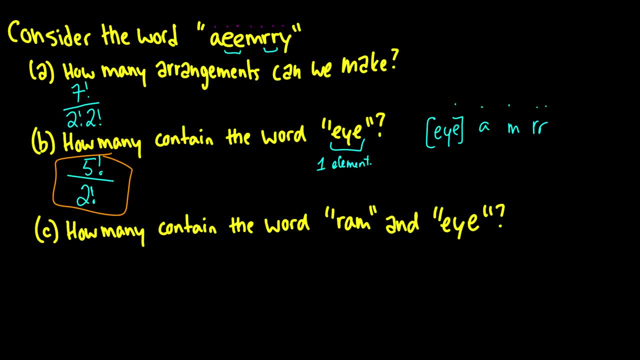 How many contain the word RAM and I? Well, again, what we do is we take the word RAM, we take the word I, and then we take the remaining letters, One letter which is going to be an R, and then we order it. 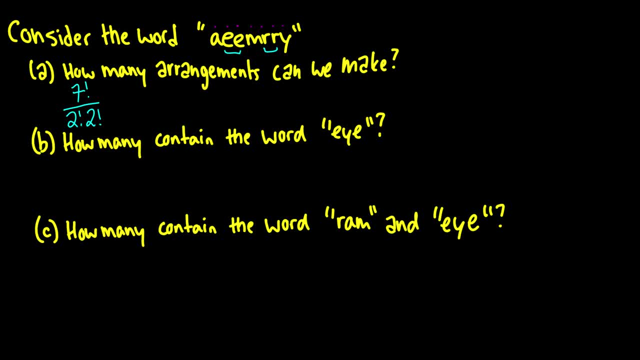 How many contain the word i. Well, now, what we do here is we take our word out. So let's take the word i out and then list the remaining letters. here We have a, we have an m and we have two r's. 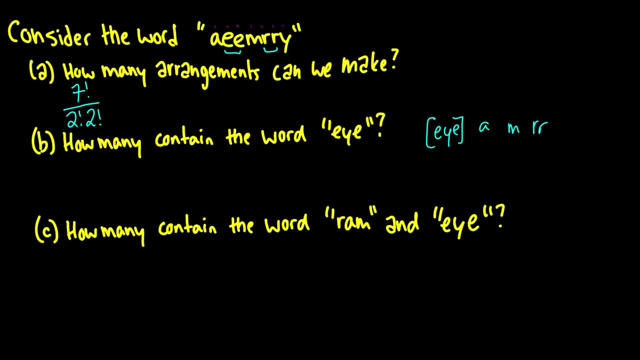 So what we do is we treat the word i As a single element. So now we actually have one, two, three, four, five total elements here. And how many repeats are there? Well, there are two r's, So this is five factorial over two factorial. 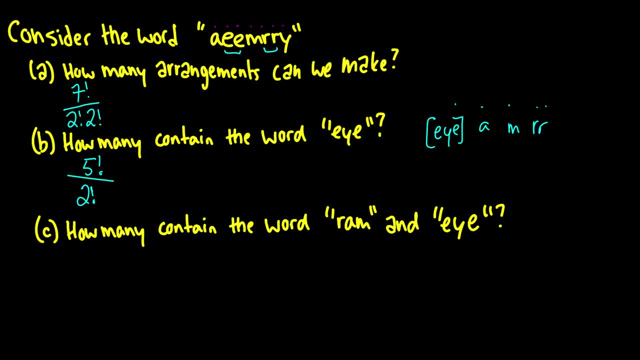 So I know this might seem a little bit confusing, But essentially we just combine the letters e, y, e into one element and then do the rest as normal. In fact, if you were to take the total arrangements and then subtract all the arrangements where 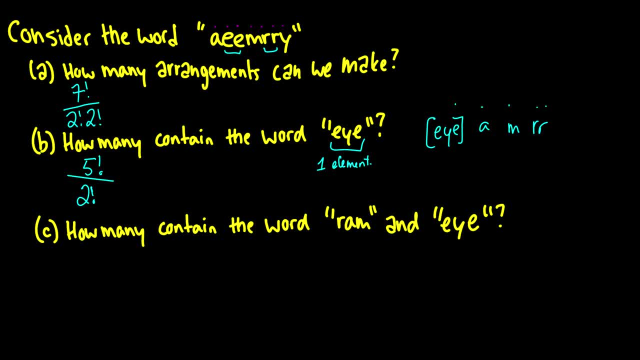 e, y, e happened to be together with much more complicated mathematics. you would end up at this same result if you did it correctly. So here's a better question: How many contain the word ram and i? Well, again, what we do is we take the word ram, we take the word i and then we take 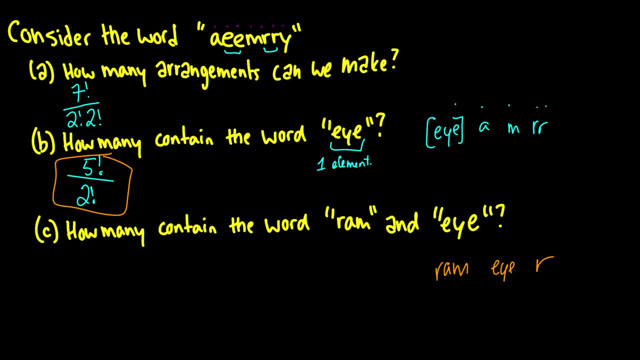 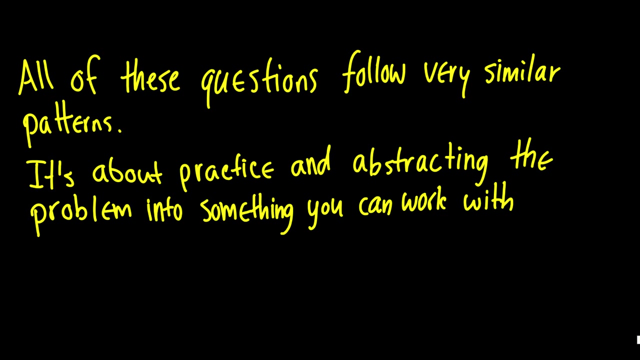 the remaining letters: One letter which is going to be an r, and then we order it. So this is going to be three factorial. So really this wasn't actually too bad of a question. Of course, what you'll notice is that all of these questions follow very similar patterns. 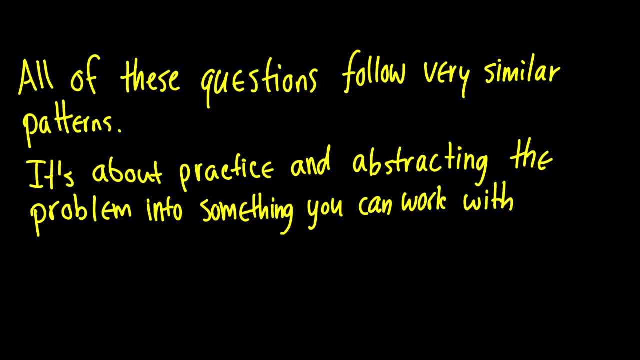 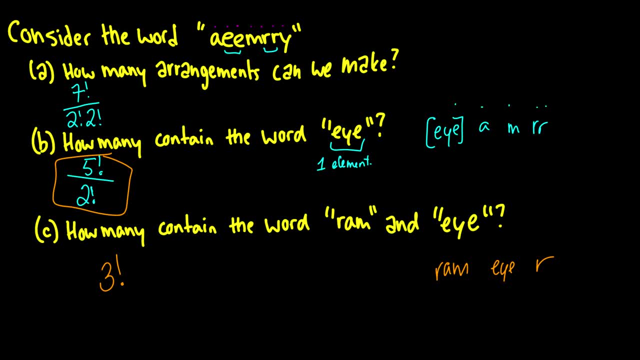 And it's really about practice and abstracting The problem into something you can work with. So you can see here in the question containing the word ram and i: well, what we just did was we did the same thing as we did with part a, except we simply put the words as a single. 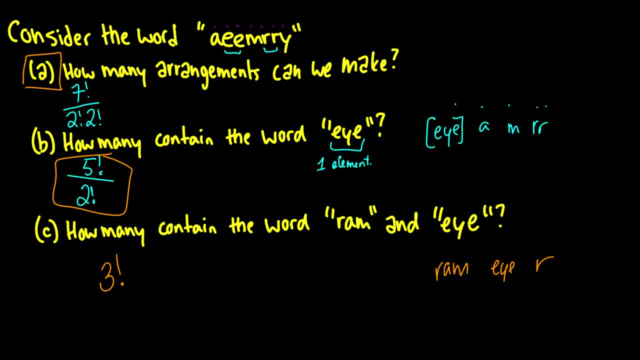 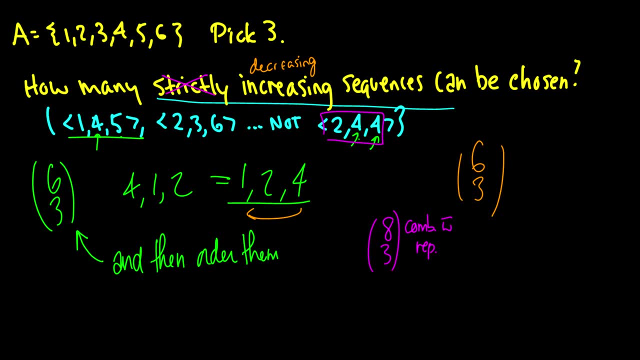 unit And we worked with them and we figured out what we could do With the question of strictly increasing sequences. well, we played around a little bit and we saw that, hey, If we took any combination, we can order it into a strictly increasing set. 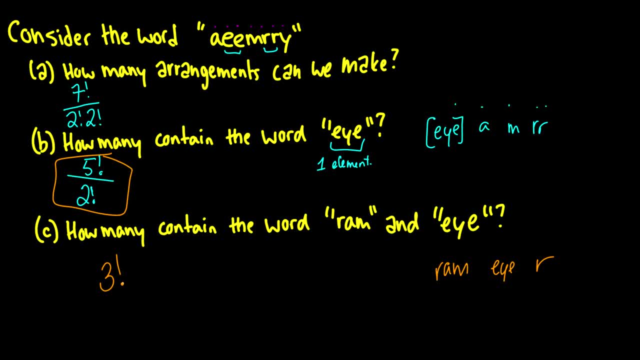 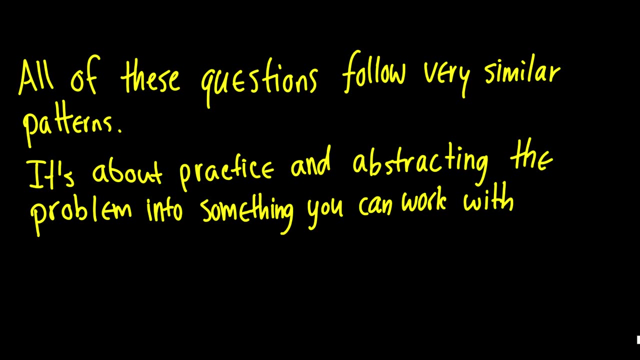 So this is going to be three factorial, So really this wasn't actually too bad of a question. Of course, what you'll notice is that all of these questions follow very similar patterns, and it's really about practice and abstracting the problem. 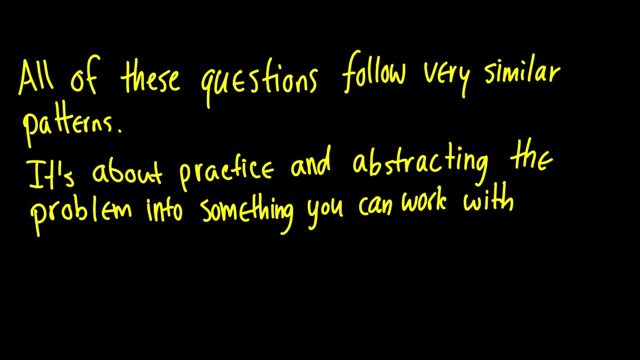 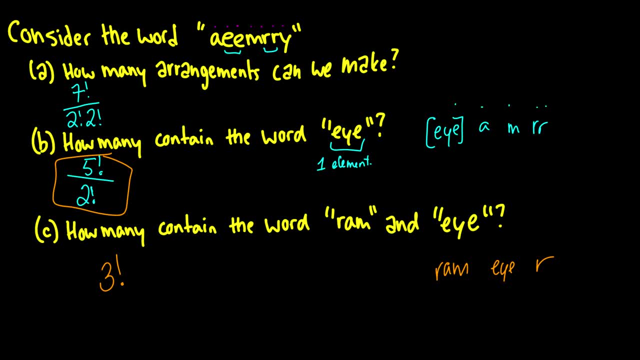 So you can see here in the question containing the word RAM and I. well, what we just did was we did the same thing as we did with part A, except we simply put the words as a single unit and we worked with them and we figured out what we could do. 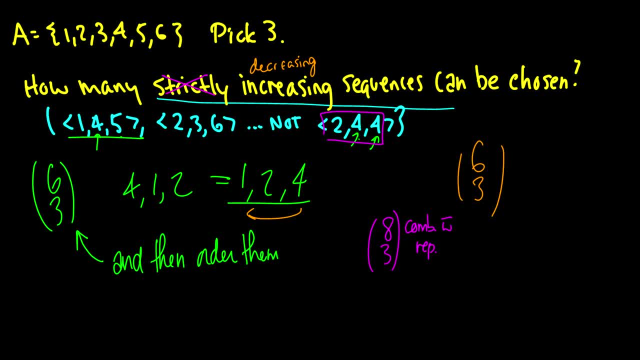 With the question of strictly increasing sequences. well, we played around a little bit and we saw that, hey Well, if we took any combination, we can order it into a strictly increasing set. So why do we have to do anything fancy? 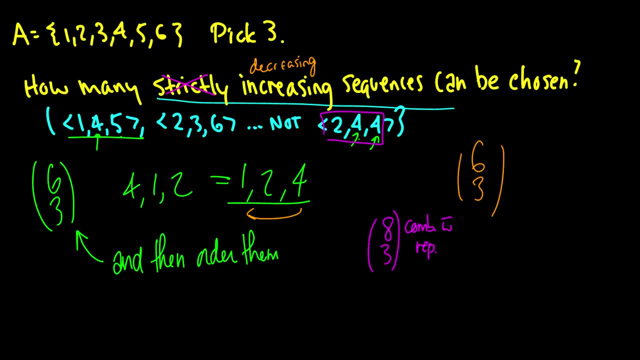 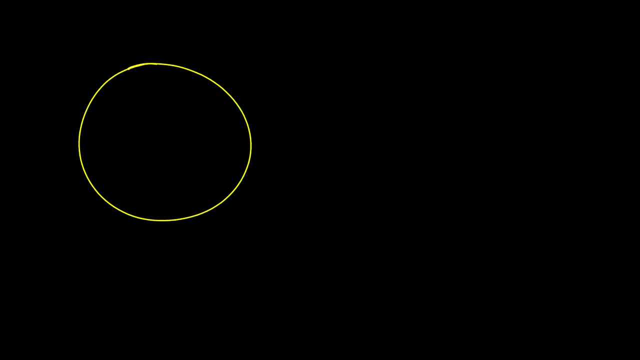 Why do we have to do cases on that? Think about the question with the round table. So, if you remember, the round table has a bunch of people, can have, say, six people sitting around a table and you think how many ways are there to arrange them. well, 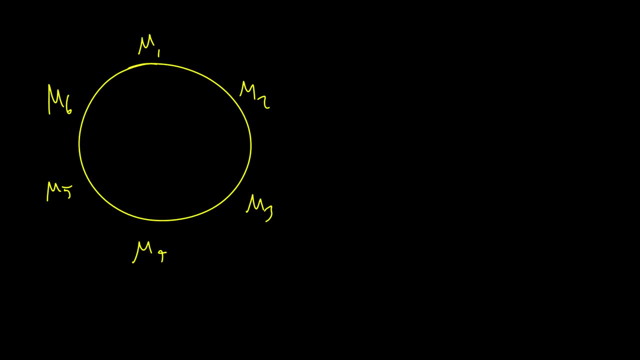 it's kind of a tricky question, But you just do the same thing as you did before, you have OK. well, there's six ways, five ways, four ways, three ways, two ways, one way, and that seems like a good answer. 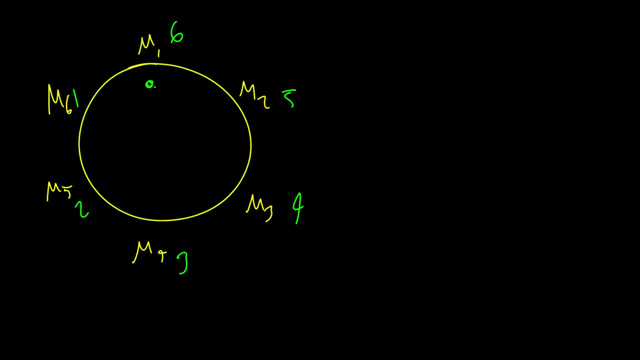 but hold on, If we rotate everyone exactly one position, it's going to be the same way. So we have to divide by six total seating positions or six rotations, and that's how you get your answer. So if you want to use that as a reference for the circular table, OK. and what if I? 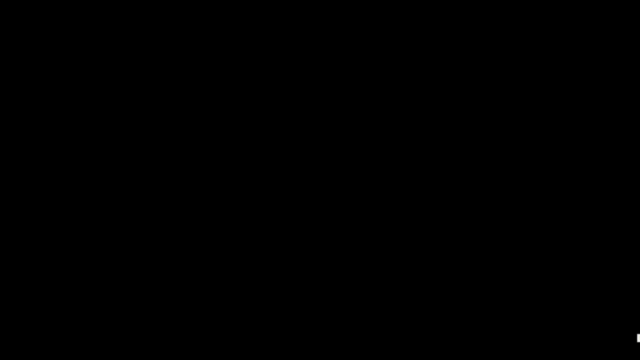 said: OK well, I have 12 books and I need to give them to four children. How do I distribute that? Well, here's another crazy thing that translates to an integer problem. OK, well, we have four children. 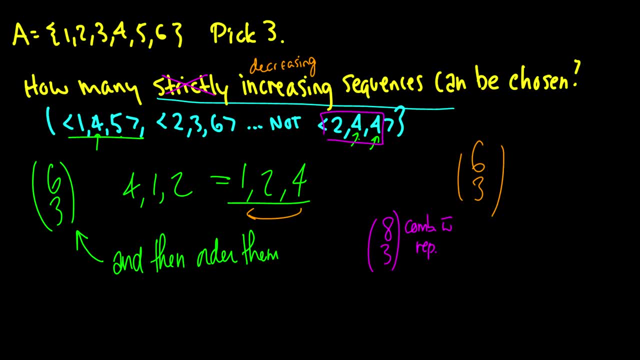 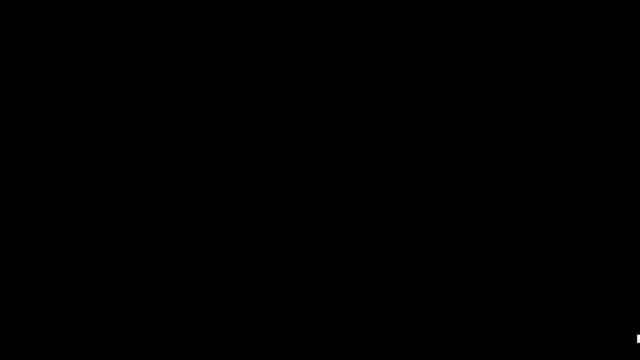 So why do we have to do anything fancy? Why do we have to do cases on that? Think about the question with the round table. So if you remember, the round table has a bunch of people- can have say, six people sitting around a table and you think how many ways are there to arrange them? 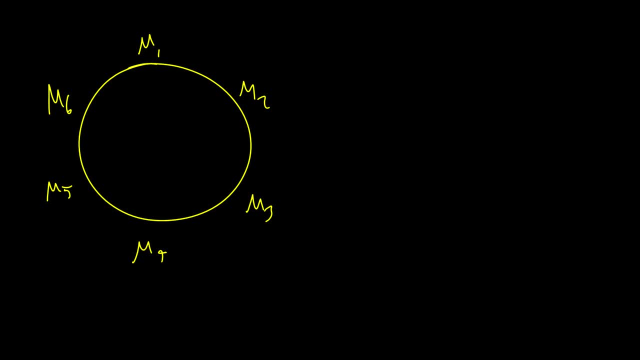 Well, It's kind of a tricky question. Yeah, It's a tricky question, but you just do the same thing as you did before. You have okay. well, there's six ways, five ways, four ways, three ways, two ways, one. 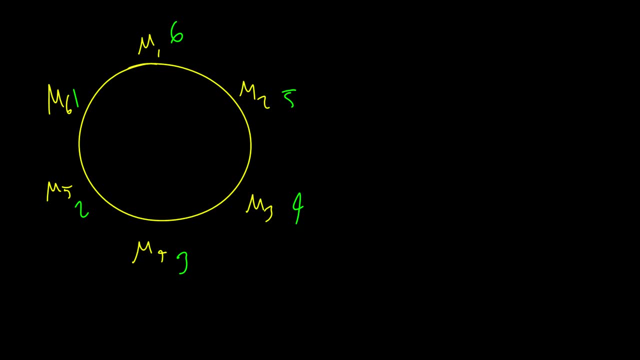 way And that seems like a good answer. but hold on, If we rotate everyone exactly one position, it's going to be the same way. So we have to divide by six total seating positions or six rotations, And that's how you get your answer for the question. 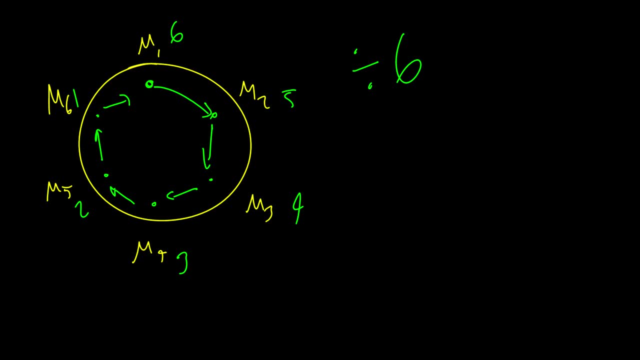 And that's how you get your answer for the circular table. Okay, and what if I said, okay, well, I have 12 books and I need to give them to four children. How do I distribute that? Well, here's another crazy thing that translates to an integer problem. 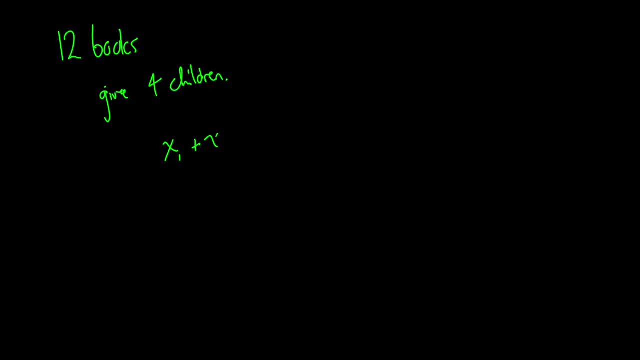 Okay, well, we have four children. X1 plus X2 equals X3.. Okay, X1 plus X2 plus X3 plus X4 is equal to 12, and now we just find the number solution to this problem. It's kind of like saying: okay, how many ways can I put 12 balls into four bins? 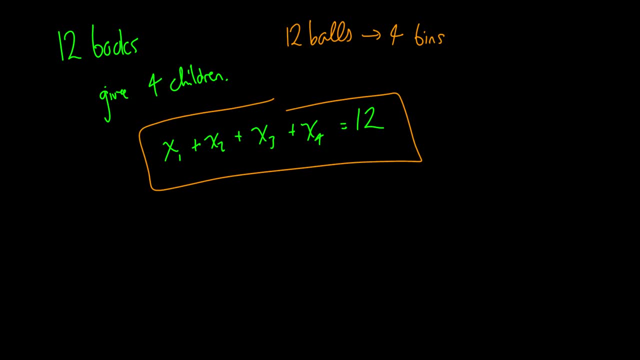 But instead of balls and bins, I'm working with books and children And of course, if you remember, this is going to be 15. choose 12 after the formula. So it's about taking what you know, seeing the problem and abstracting it into something. 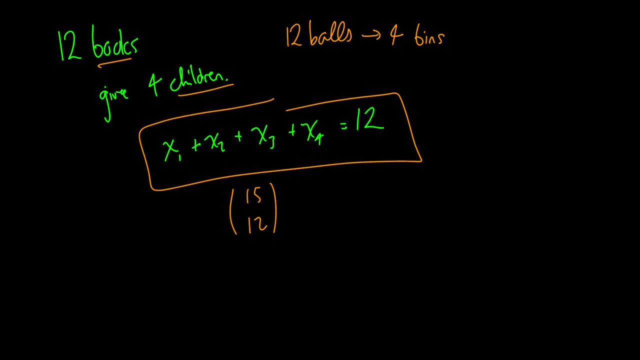 that you know how to work with. So there's tons of practice problems online. The ones I gave you here are the basic problems you're going to see in an exam. You're not going to get that much harder And I did a lot of practice problems in the previous videos and I don't think you'll 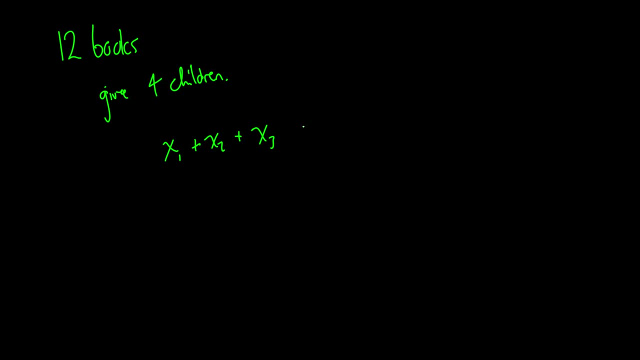 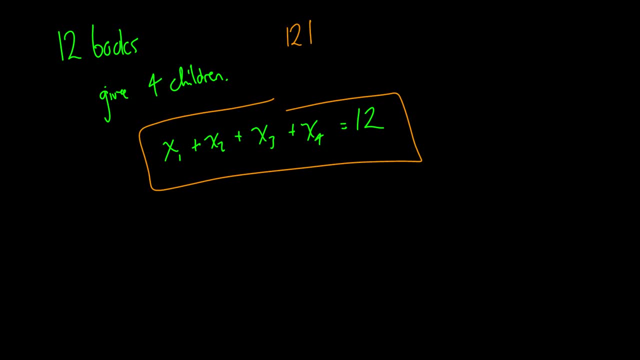 It's kind of like saying: okay, how many ways can I put 12 balls into 4 bins? But instead of balls and bins, I'm working with books and children And, of course, if you remember, this is going to be. 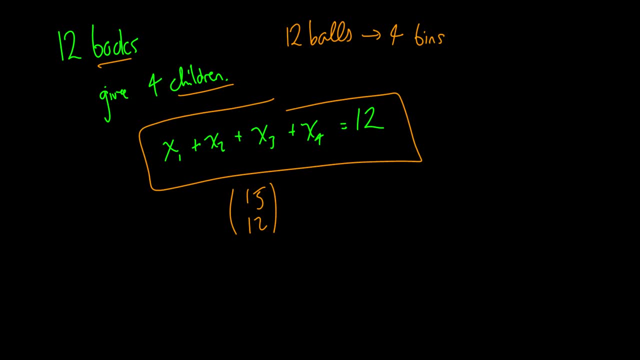 15, choose 12 after the formula. So it's about taking what you know, seeing the problem and abstracting it into something that you know how to work with. So there's tons of practice problems online. The ones I gave you here are the basic problems you're going to see in an exam. 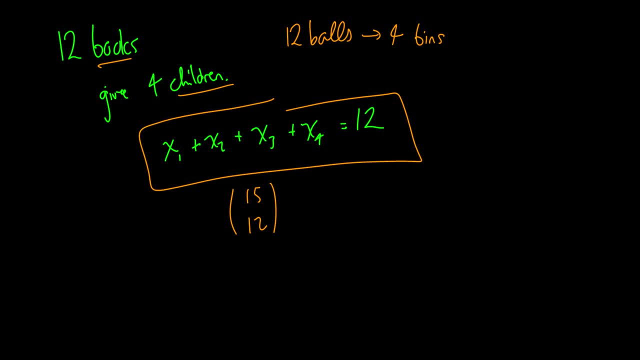 They're not going to get that much harder, And I did a lot of practice problems in the previous videos, and I don't think you'll see anything outside of that, unless your professor has specifically designed it for you. So I'm going to show you how to do that. 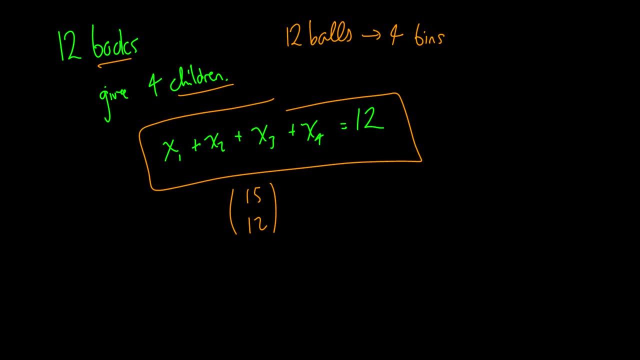 I'm going to introduce some different type of problem in lecture, in which case, learn that and abstract it. You need to take this stuff to a very abstract level if you want to succeed. The best way to understand discrete math is to take a bunch of example. 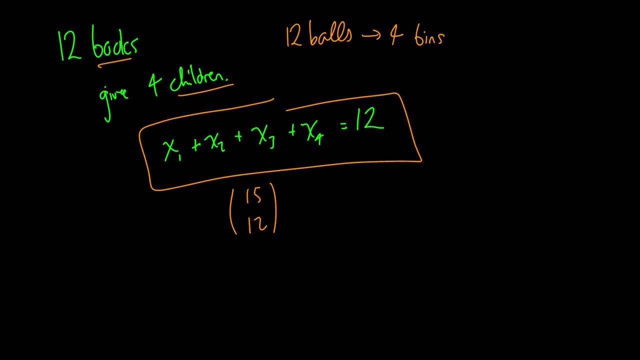 questions and see how they're all related and translate them into one common thing, For instance, combination with repetition. turn every question into an integer question like this. I'm putting tons of arrows in here, because this is the key to all questions that involve combinations with repetitions. You turn it into this bad boy and you will be safe for life. 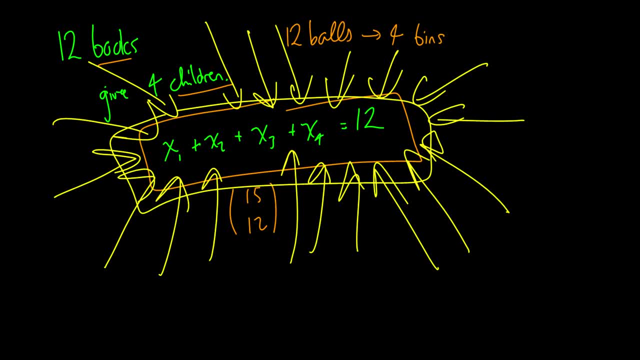 You will understand combinations with repetitions once you understand how this integer solution works and are able to translate everything to an integer solution question. This is my key tip for discrete math. if you haven't figured it out yet: Abstract everything. Abstraction is the key to success, and that is my rant, or lecture. 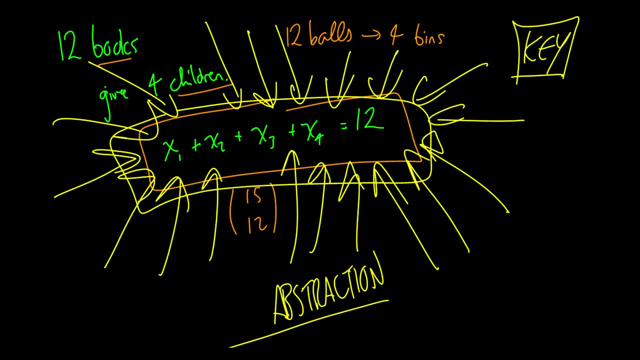 I guess when you watch an education video, a rant really is just a lecture. so I mean, hey, it sounds better if I put it on like a resume or something, instead of saying, oh, yeah, rants at children. It's like: no, no, I lecture at children. You guys aren't children. 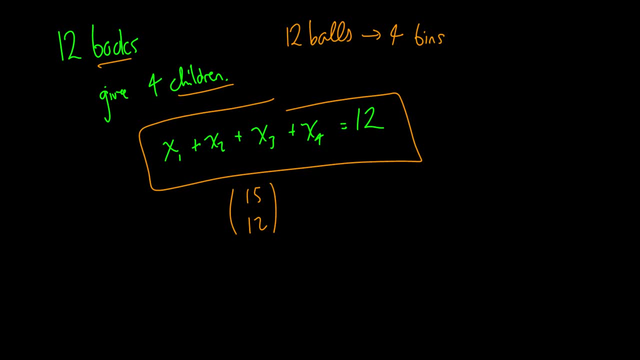 see anything outside of that, unless your professor has specifically introduced some different type of problem in lecture, In which case let's go back to the problem. Let's go back to the problem, Learn that and abstract it. You need to take this stuff to a very abstract level if you want to succeed. 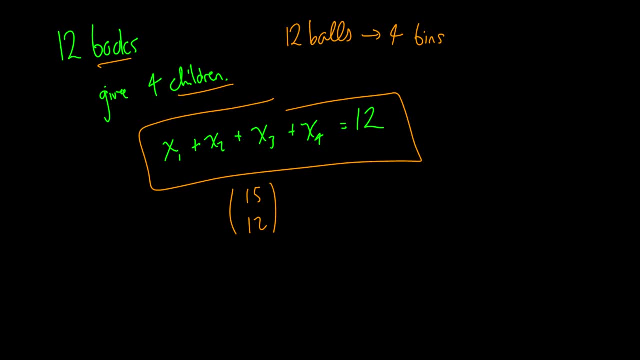 The best way to understand discrete math is to take a bunch of example questions and see how they're all related and translate them into one common thing. For instance, combination with repetition. turn every question into an integer question like this. I'm putting tons of arrows in here. 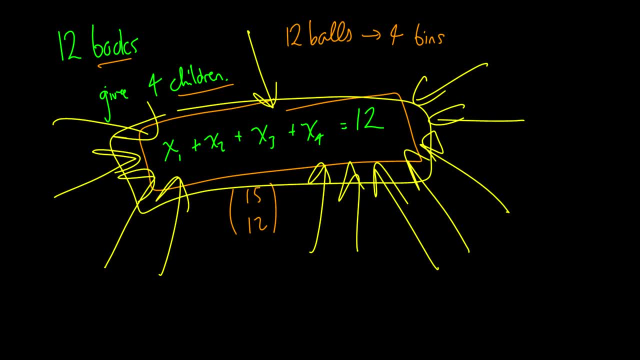 This is the key to all questions that involve combinations with repetitions. You turn it into this bad boy and you will be safe for life. You will understand combinations with repetitions once you understand how this integer solution works and are able to translate everything to an integer solution question. 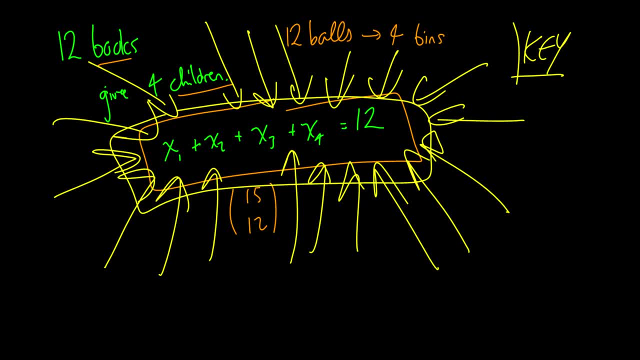 This is my key tip for discrete math. if you haven't figured it out yet: Abstract everything. Abstraction is the key Counting is the key Counting is the key Counting is the key to success, And that is my rant. 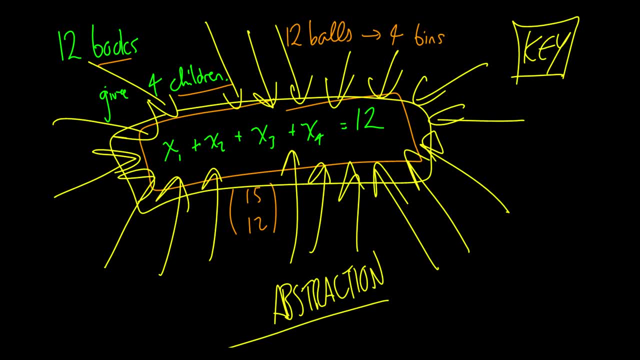 Or lecture. I guess when you watch an education video, a rant really is just a lecture. So I mean, hey, it sounds better if I put it on like a resume or something instead of saying, oh yeah, rants at children, It's like no. 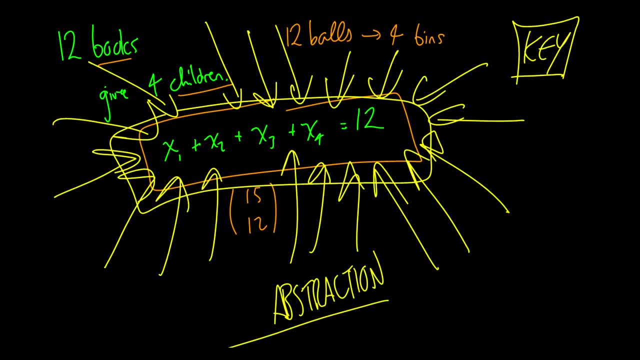 No, I lecture at children. You guys aren't children, you guys are teenagers and young adults. Anyways, that was counting practice. That is pretty much it for the counting section, At least in a few in a first level math course or discrete math. 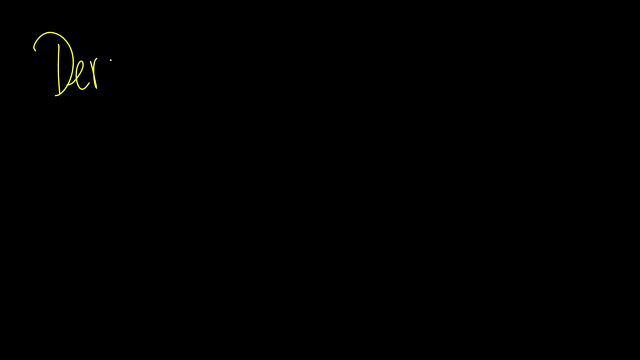 The only thing left I could do is something called derangements, but this will be covered in discrete math 2 when I ever start doing that series. So that is all that's left. Next time we start proofs- and proofs are the key component to everything math. 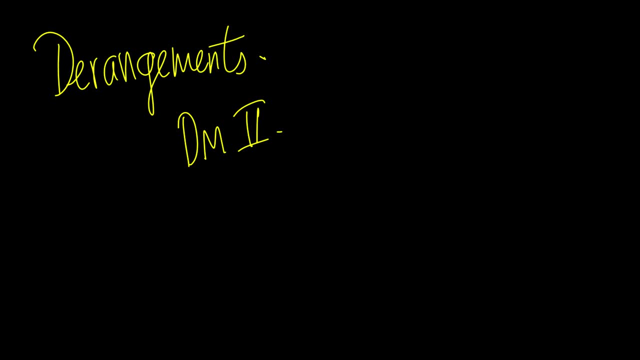 So we have a good background now and we can finally start doing some crazy proofs.